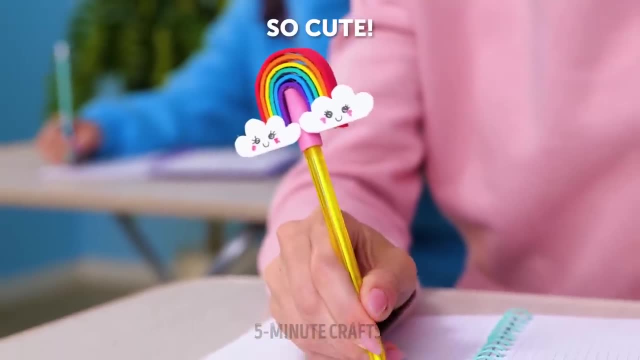 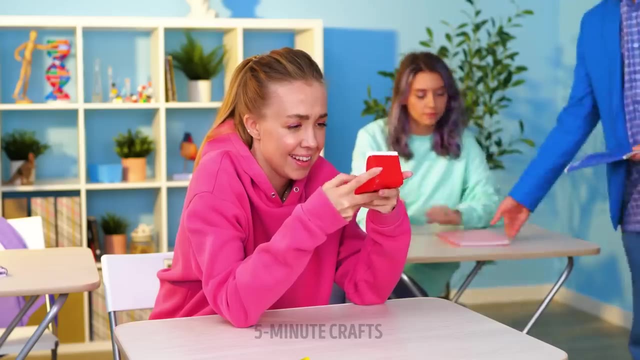 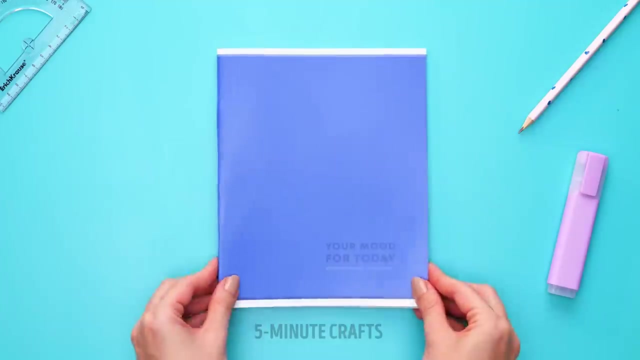 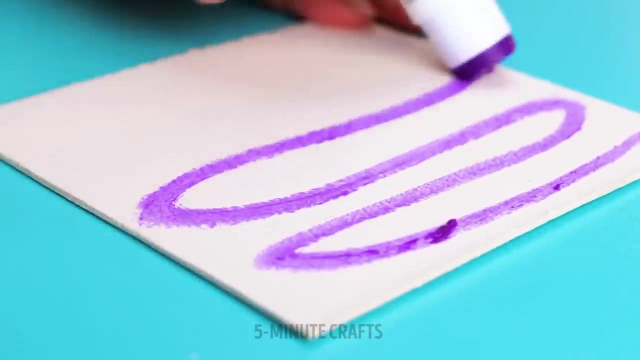 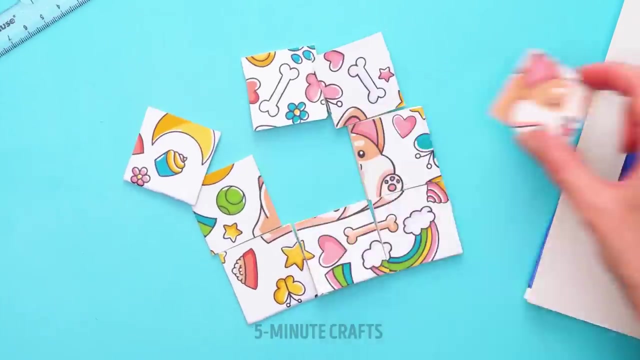 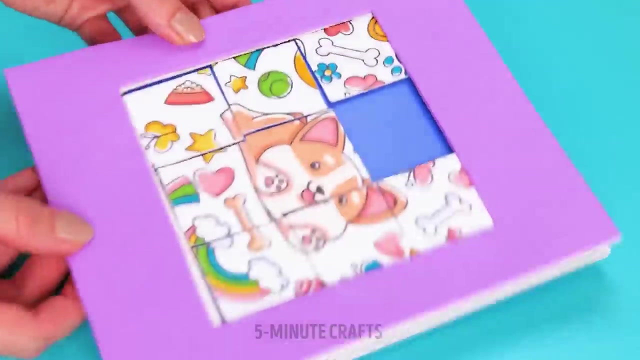 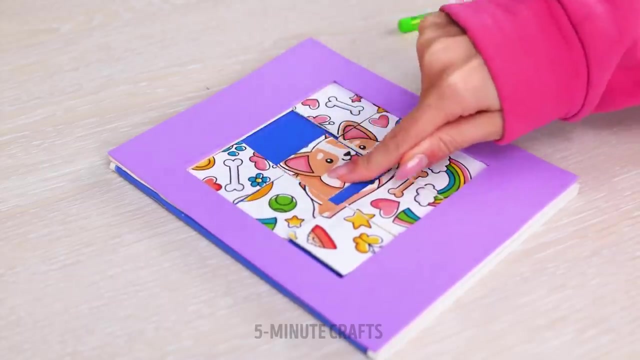 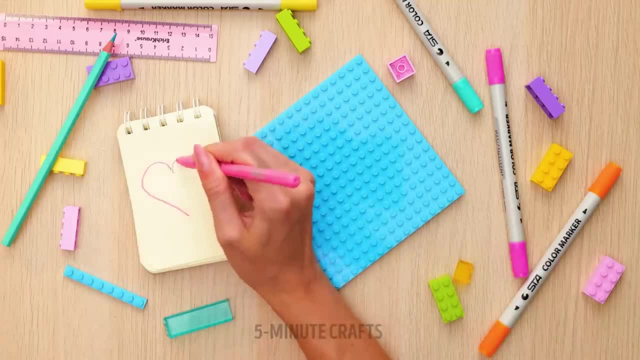 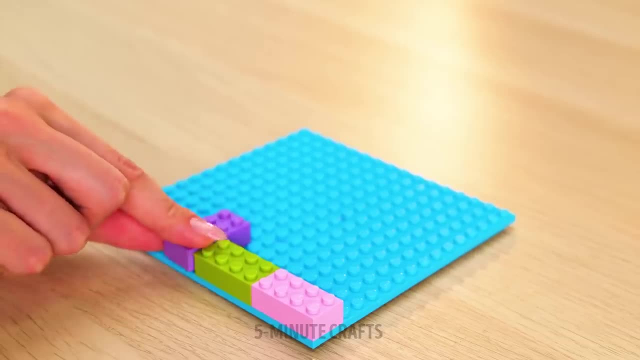 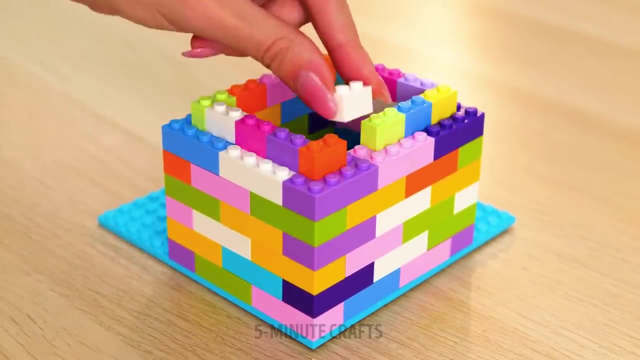 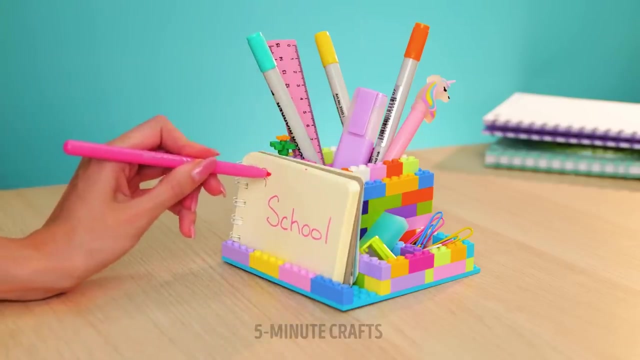 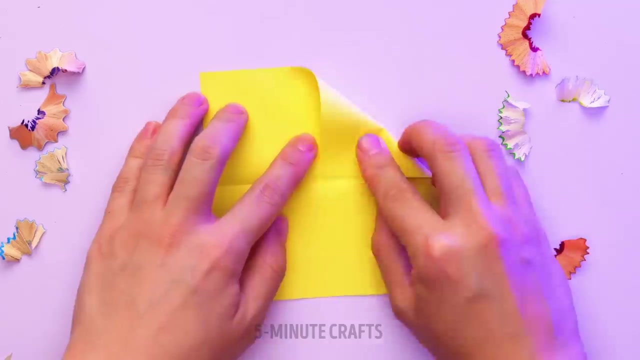 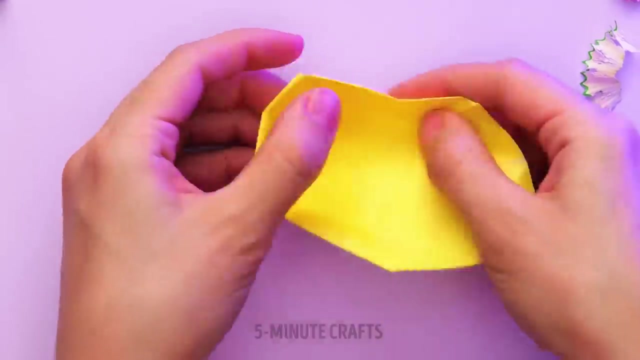 Oh baby, yes, Oh baby, yes, oh, Oh baby, yes, oh, Gotta do so, Gotta do so, Gotta do so. You have a way. it is hard to get Behind those blue eyes. are you serious? I need to know. I've tried to stay, I have tried to go. 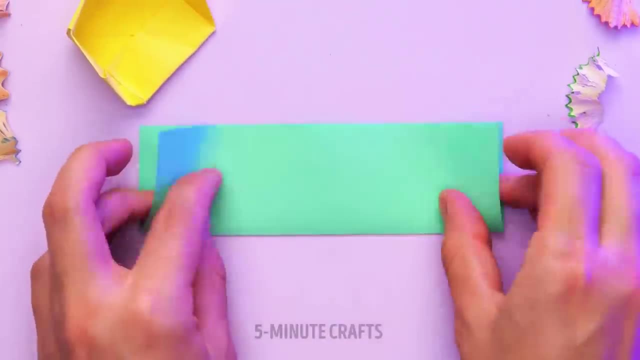 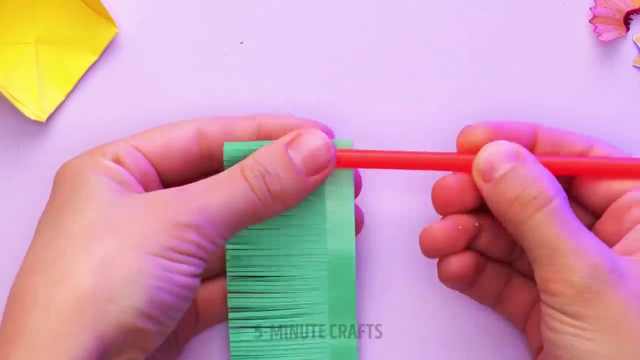 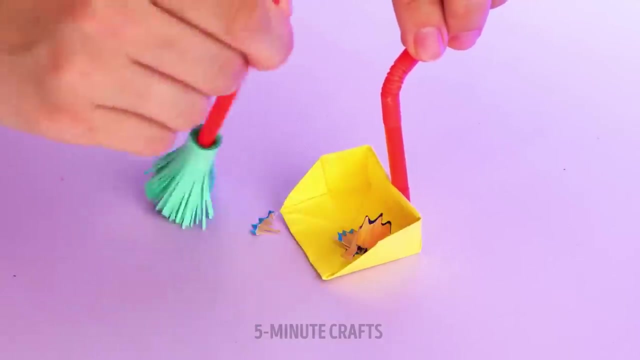 But either way, you're always in control. I need to know you're just playing. I've been waiting If you're worth my time, or am I fooling myself? You set the bar, you build it up, You start a game that needs to go. 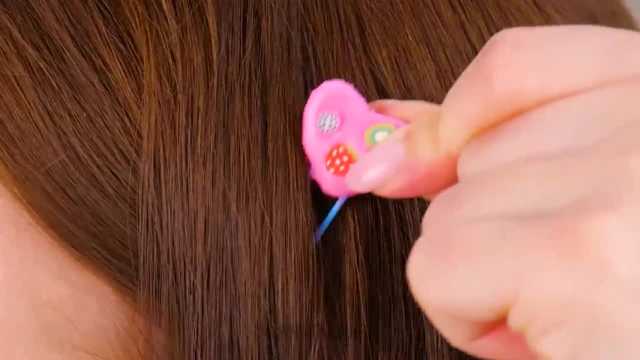 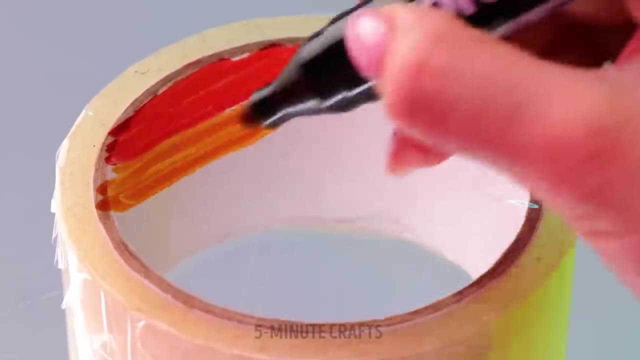 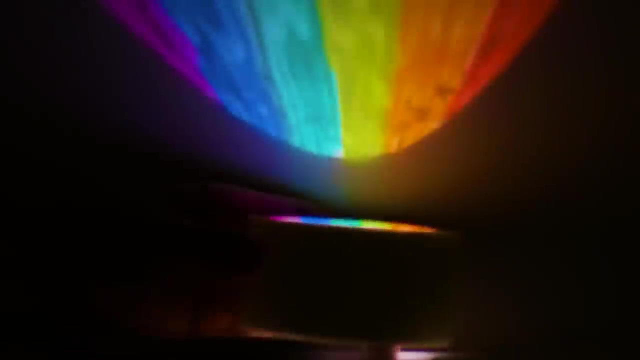 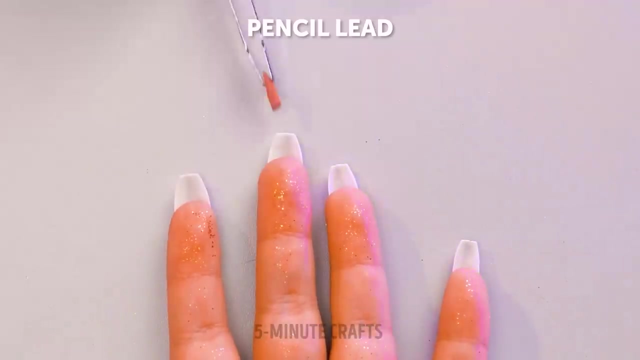 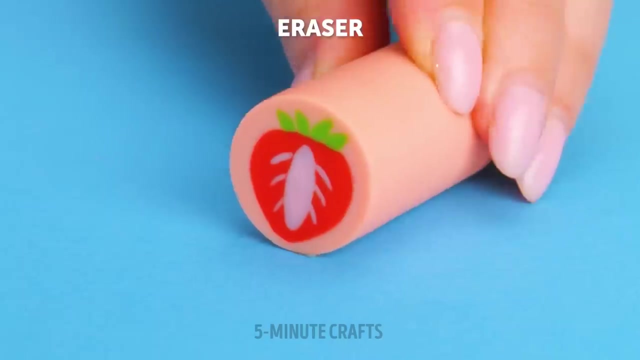 You start the fire that burns me up. Now I need your. yeah, I need your touch. Yeah, Yeah, Now I need your. yeah, I need your touch. It's 2am, you call me up, Mess with my head, but I don't need more problems. 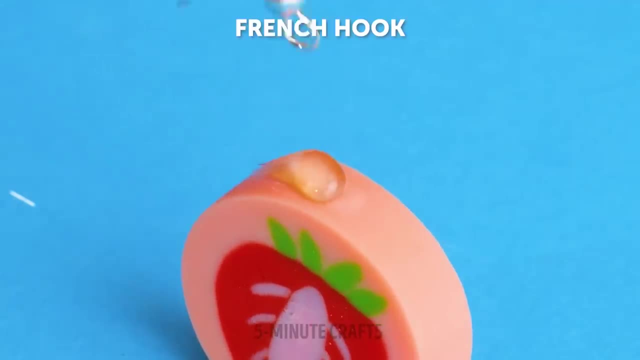 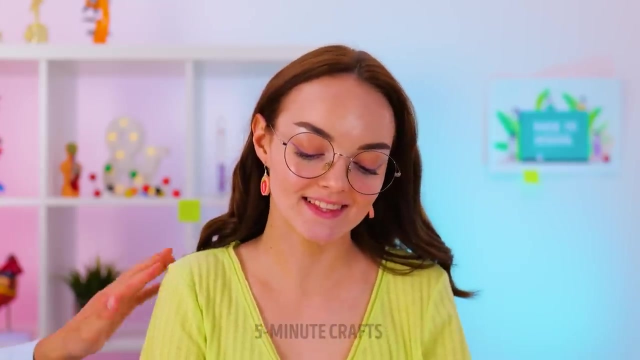 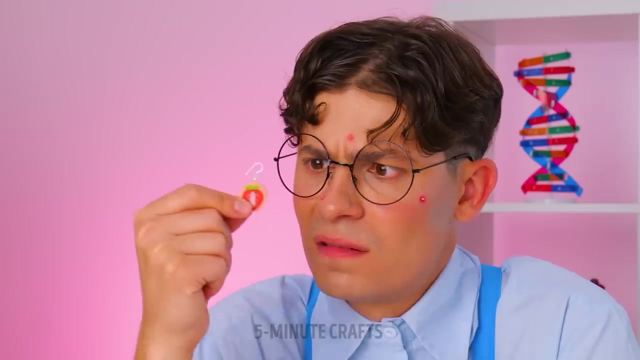 When you insist, I I can't resist You. start me up. Look in your eyes. you're always in control. I need to know you're just playing. I've been waiting If you're worth my time, or am I fooling myself? 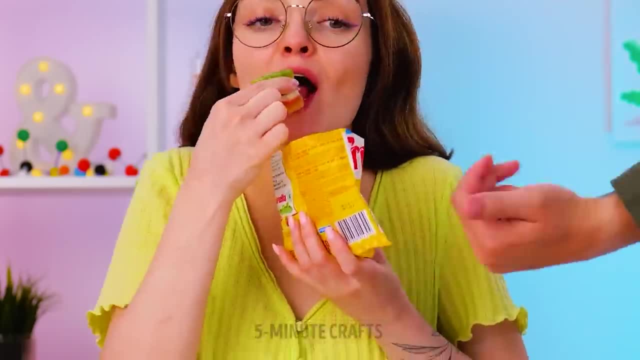 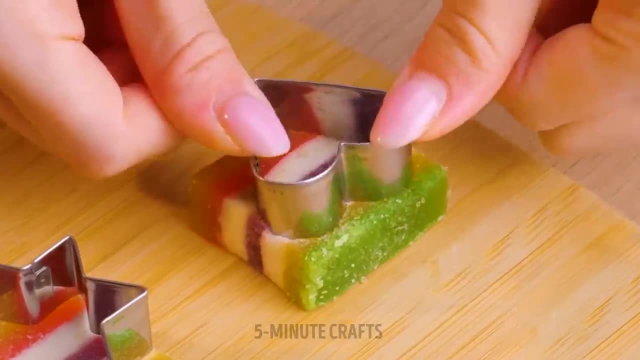 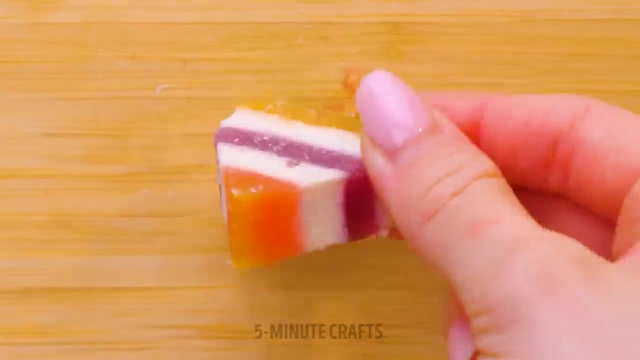 You set the bar, you build it up, You start a game that needs to go. You start the fire that burns me up. Now I need your- yeah, I need your- touch. You start the fire that burns me up. You start the fire that burns me up. 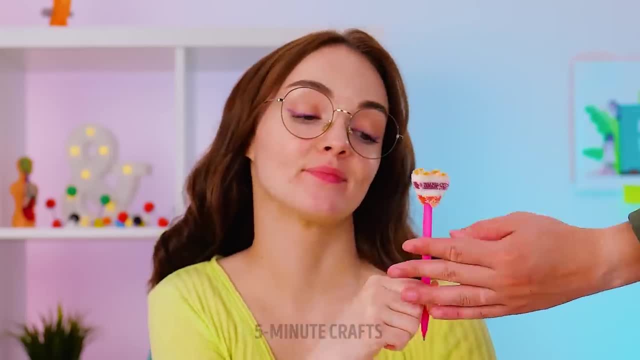 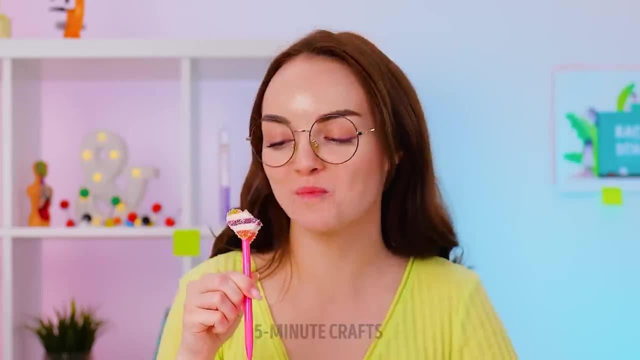 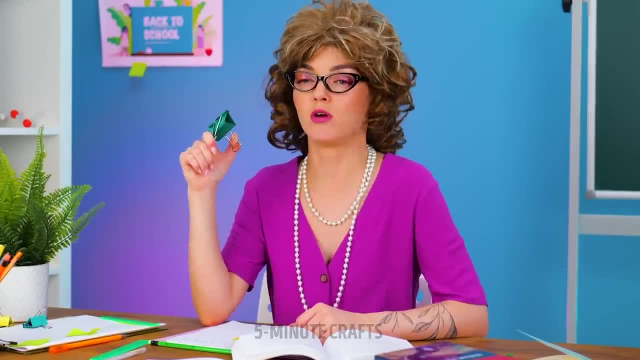 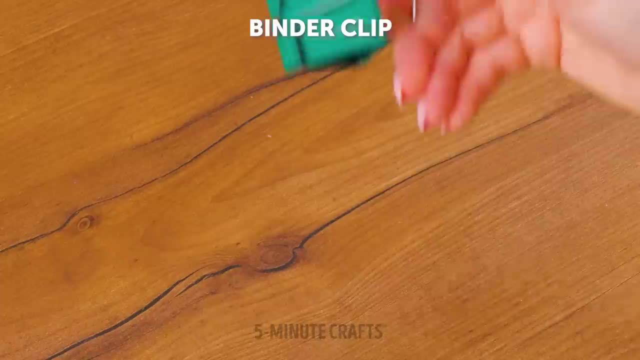 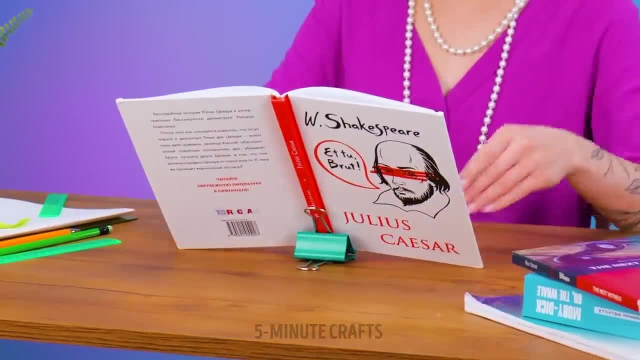 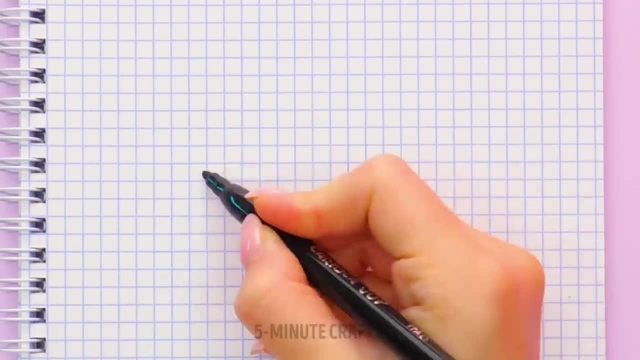 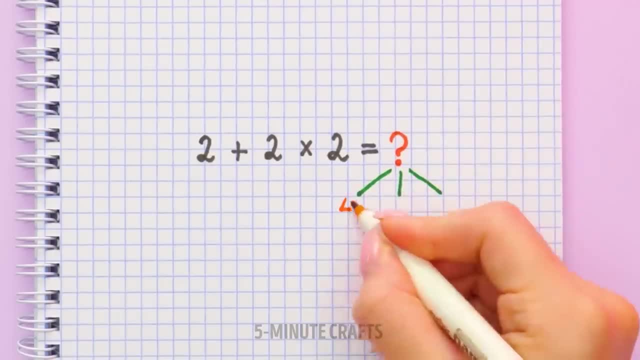 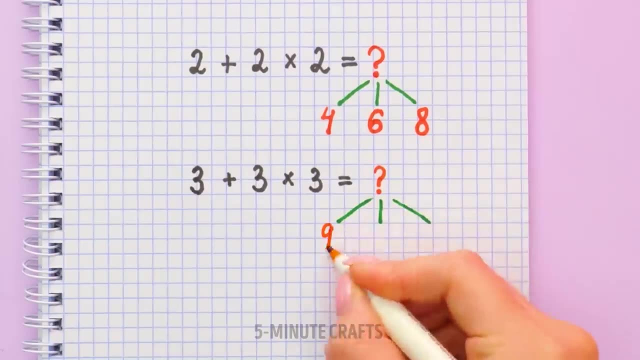 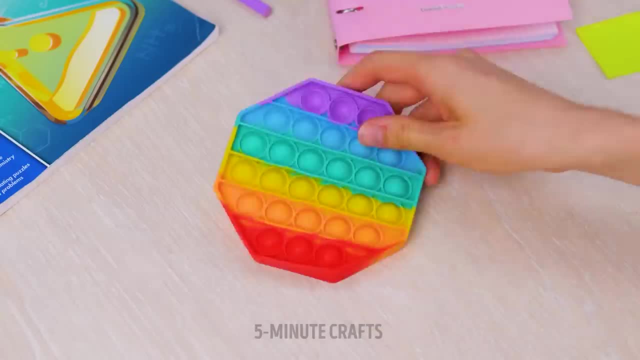 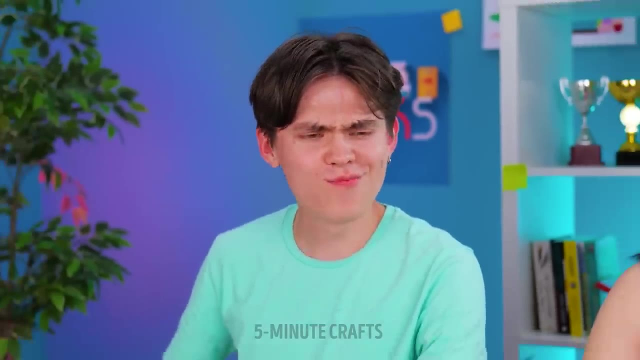 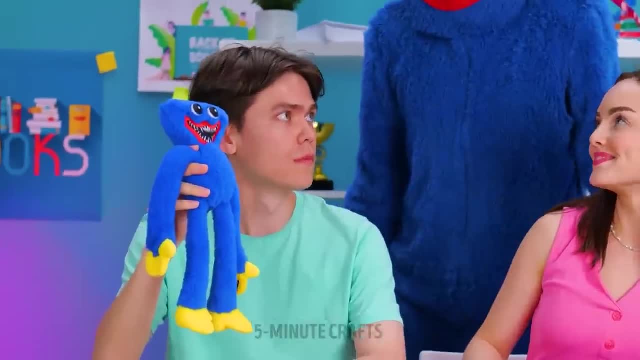 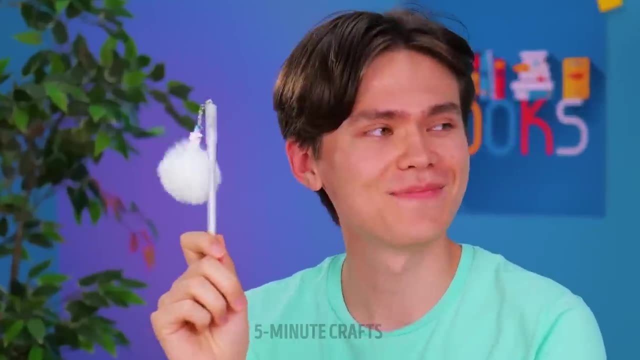 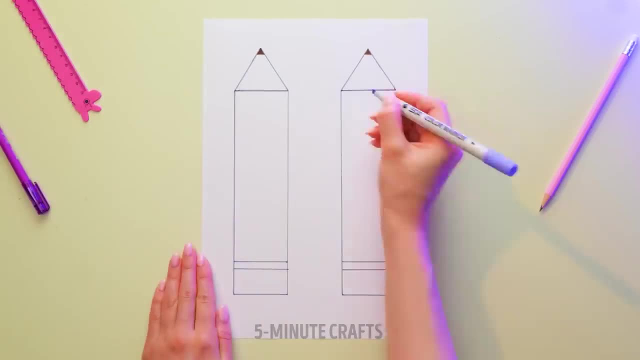 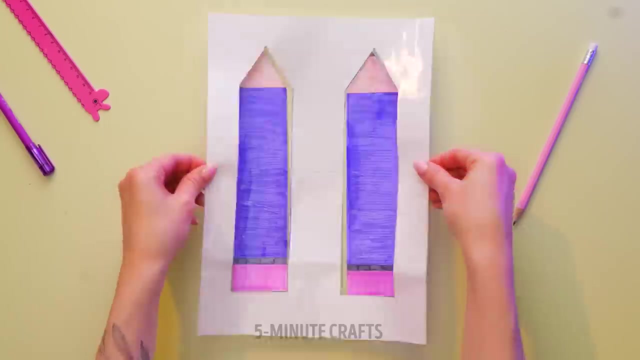 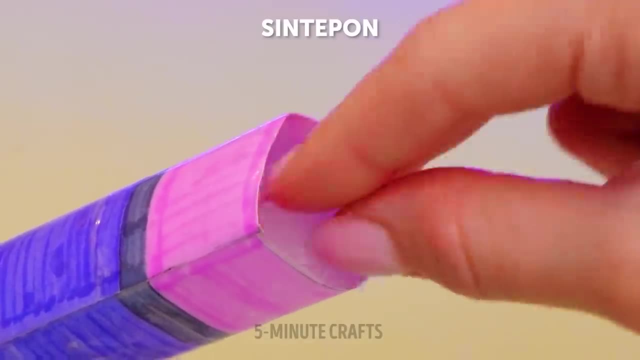 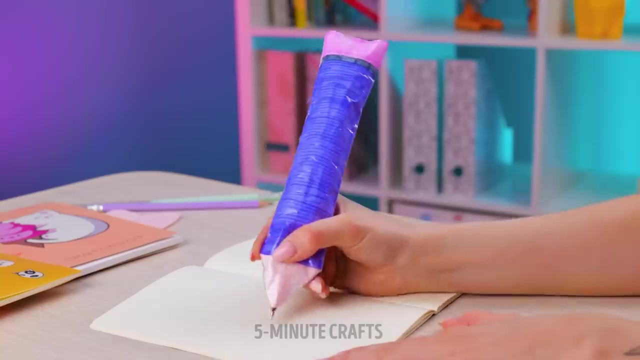 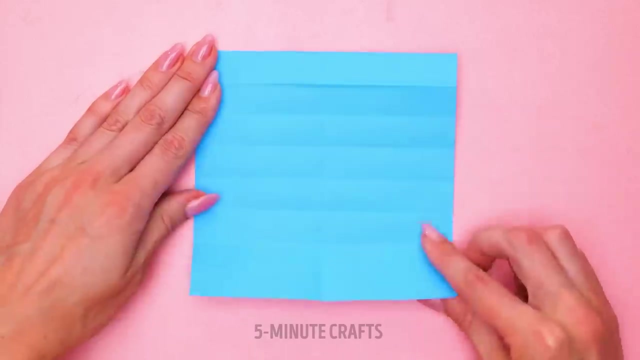 Endless love is coming. I'll be sure of that. But it's so hard Cause it's you. it's you Always on my mind. Yeah, it's you. it's you Taken all my time. Let it sink in. Haven't you been hurtin' enough? 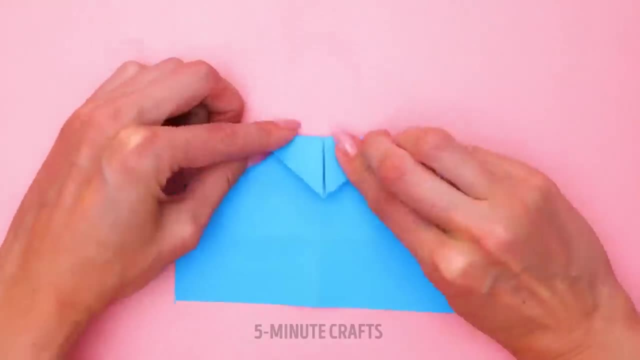 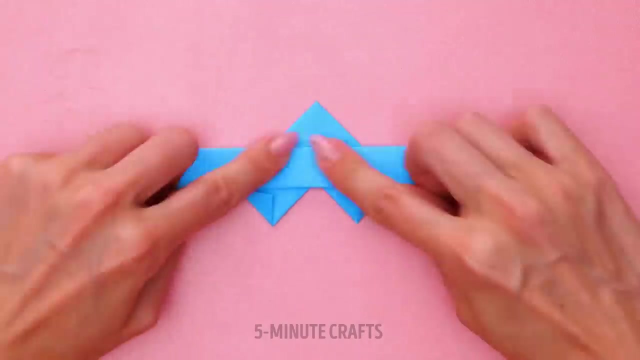 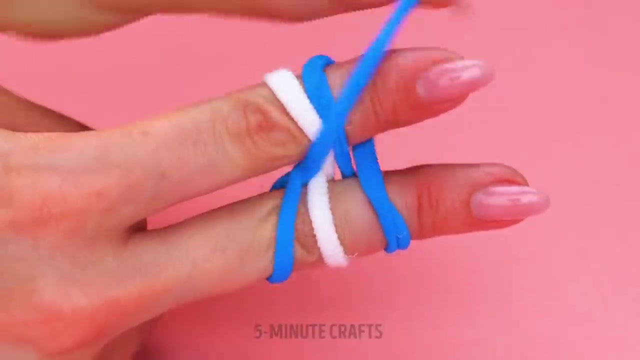 Give you all of my love. Subtitles by Levi. But you don't seem to care. But my heart's around you, But your heart isn't there. Don't tell me we're fine Lying to yourself. It's too late to meet up. We are too far apart. 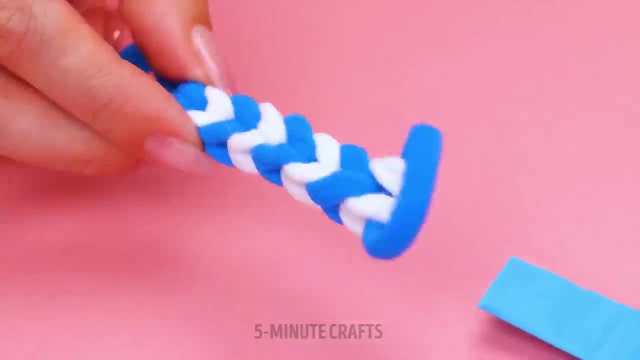 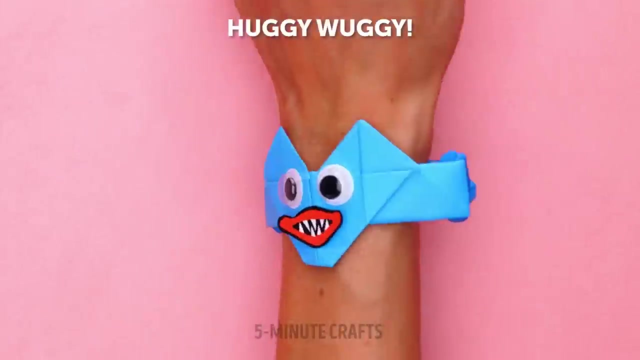 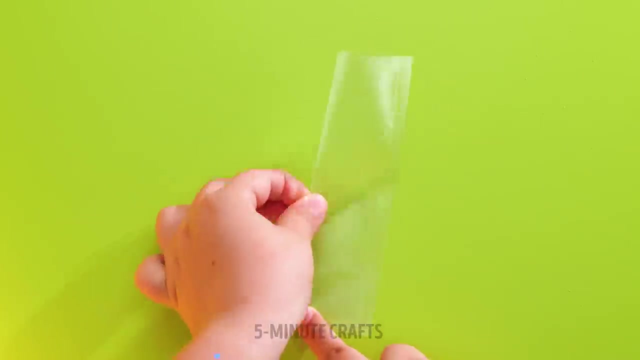 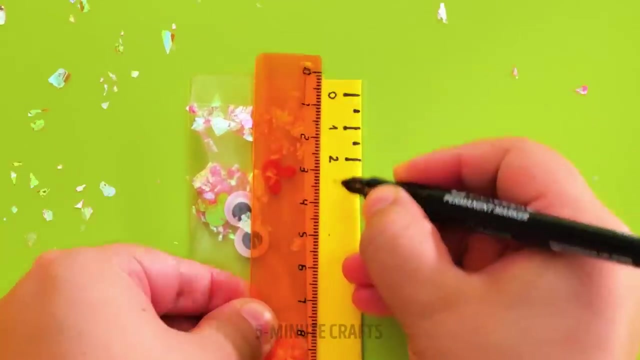 It's too late, can't you see? I can't trust you no more. Gotta get over you, Cause I'm more than the dark. It's too late to meet up. It's too late to meet up. It's too late to meet up. Don't go there. 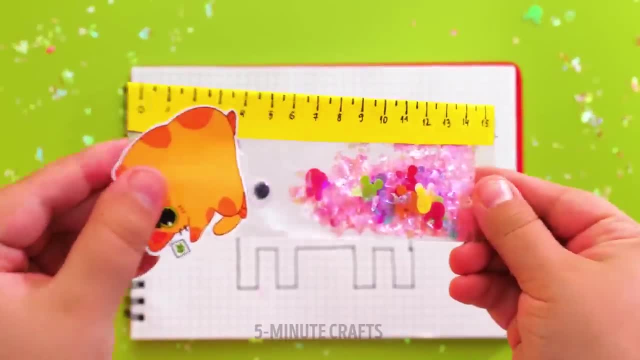 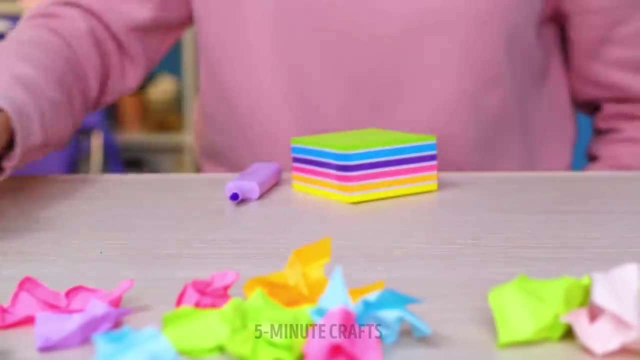 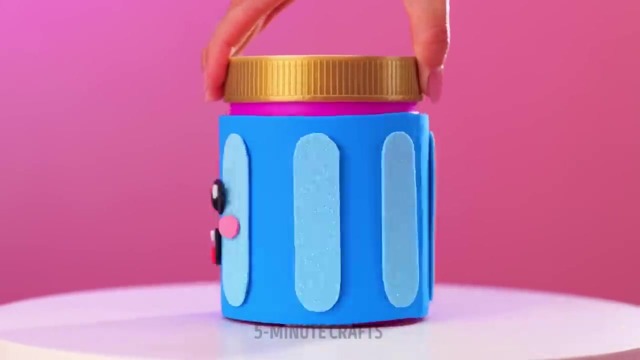 Cause you can't finish what you start. I can't keep up. You're holding back, And then you let it go too far. Just stay, Just stay, Just stay away. But it's you, it's you Always on my mind. Yeah, it's you, it's you. 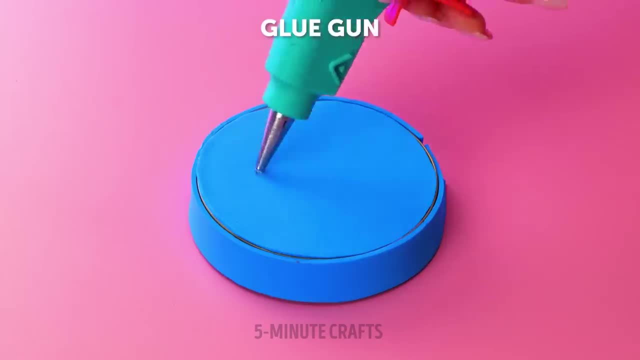 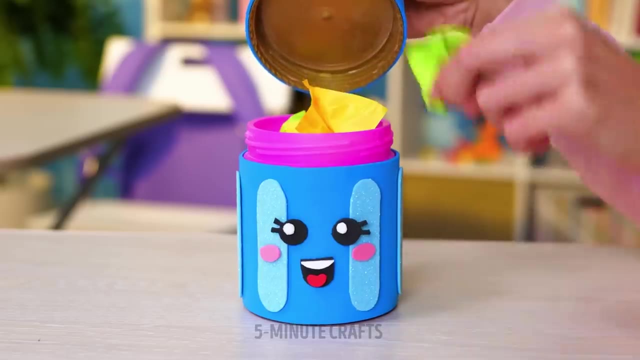 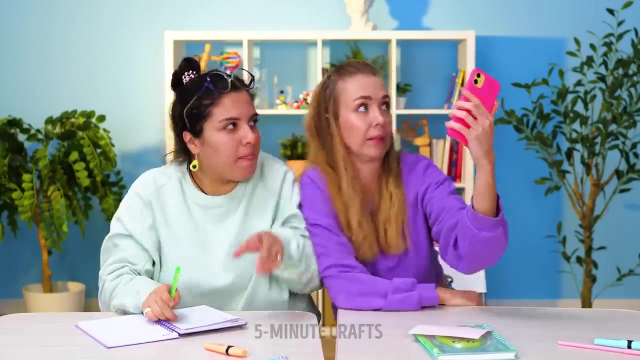 Taking up a diamond. Let it sink Heaven. I've been hurting enough. Oh oh. You are all of my love, But you don't seem to care. But my heart's around you, But your heart isn't there. Don't tell me, we're fine, Lying to myself. 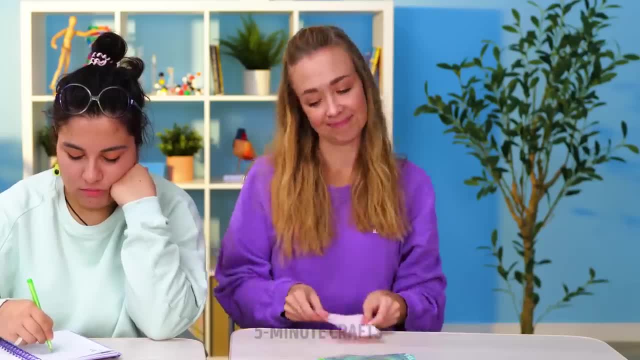 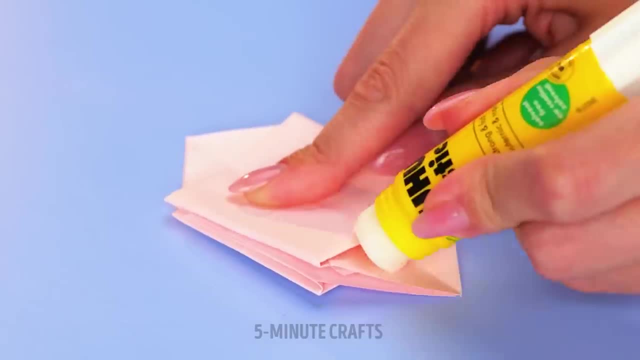 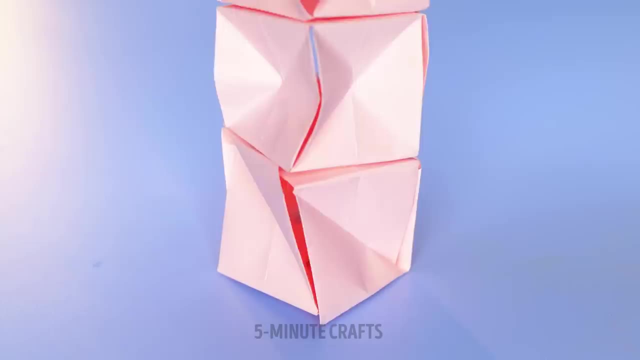 Lying to yourself. It's too late to meet up. We are too far apart. It's too late, can't you see? I can't trust you no more. Gotta get over you, Cause I'm more than the dark. It's too late to meet up. 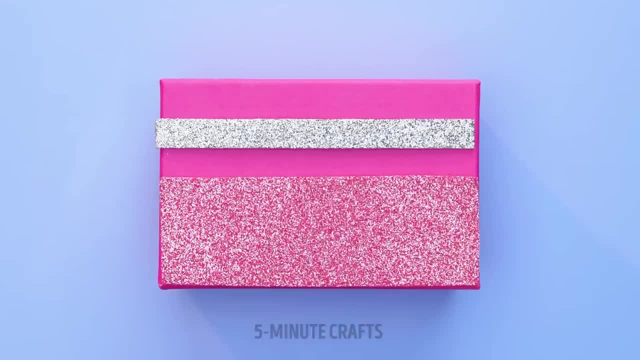 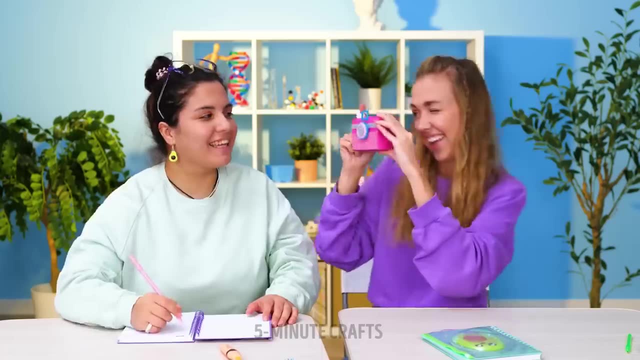 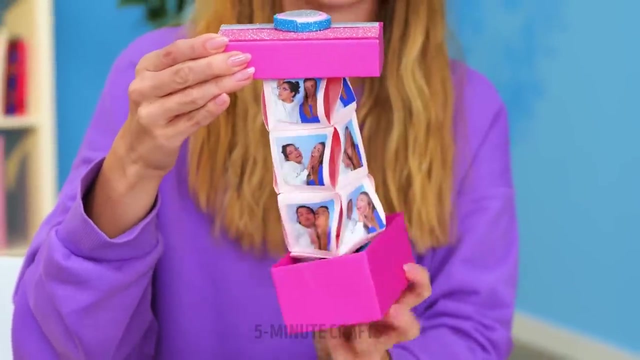 Too late to meet up. Too late to meet up. Gotta get over you, Cause I'm more than the dark. It's too late to meet up. I can't trust you no more. It's too late to meet up. Too late to meet up. It's too late to meet up. 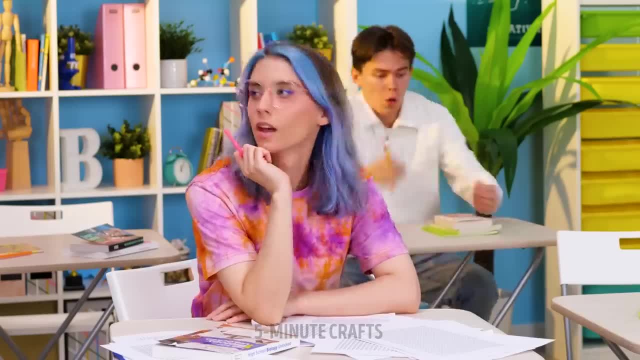 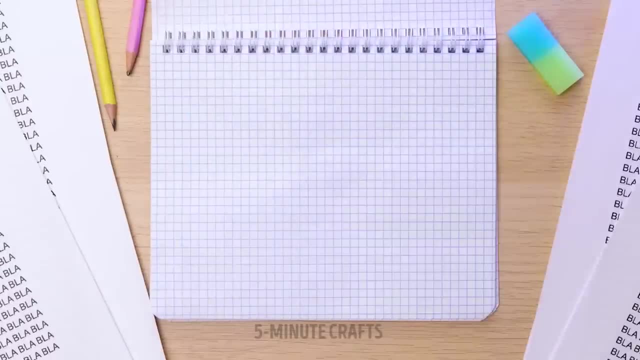 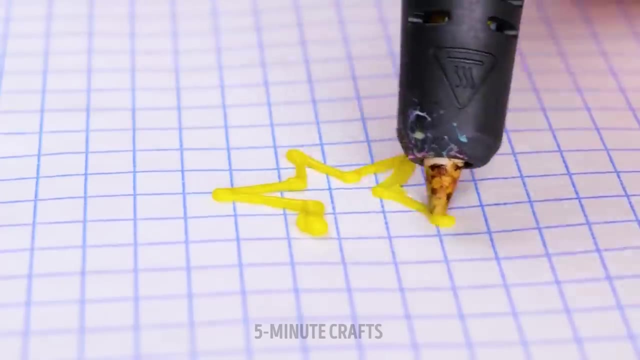 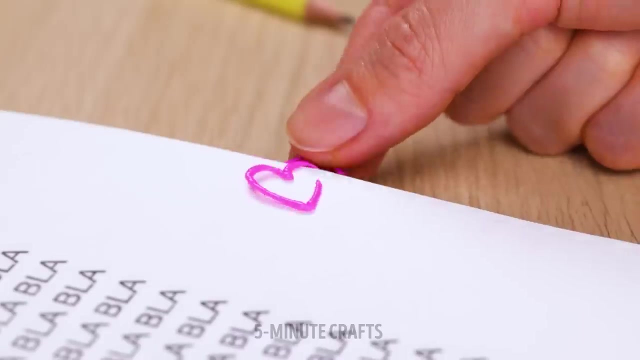 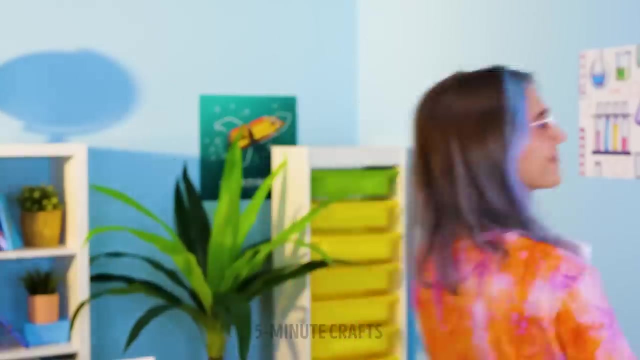 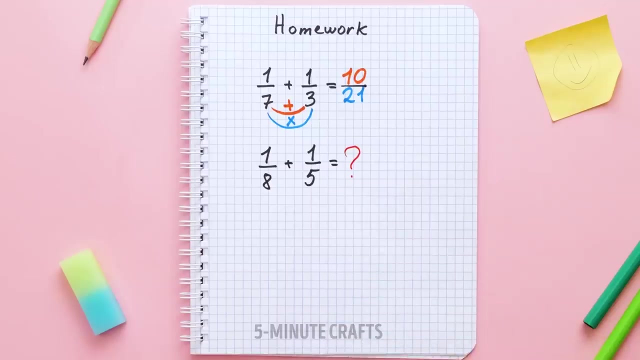 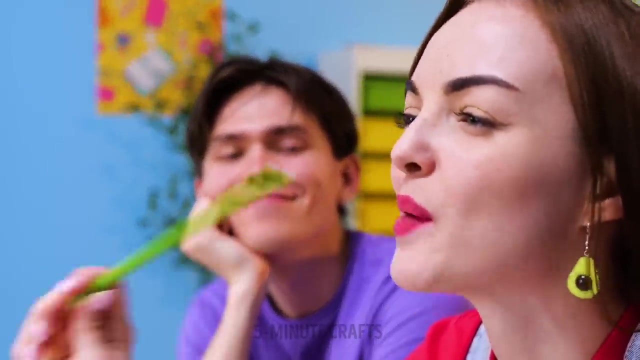